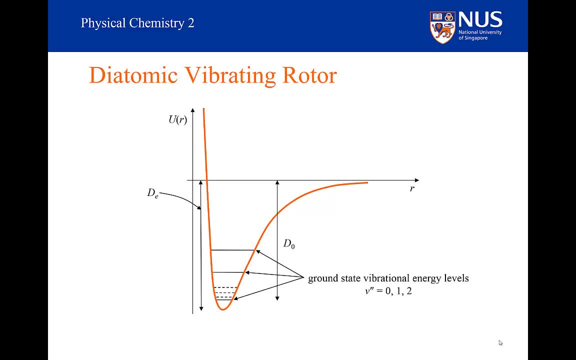 They are all defined by the quantum number- v equals zero, But they have different rotational energies. They have different values of j. Molecules, in the energy level identified by the solid line associated with v equals zero, have the vibrational energy associated with v equals zero. 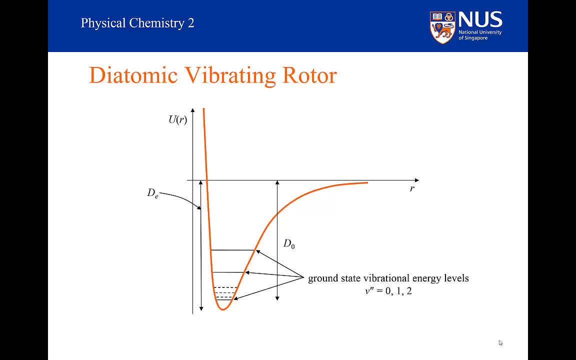 But they also have a rotational energy associated with j equals zero. Molecules in the energy levels identified by the dashed lines also have vibrational energy associated with v equals zero, But they have rotational energy associated with j equals one, j equals two, j equals three, etc. 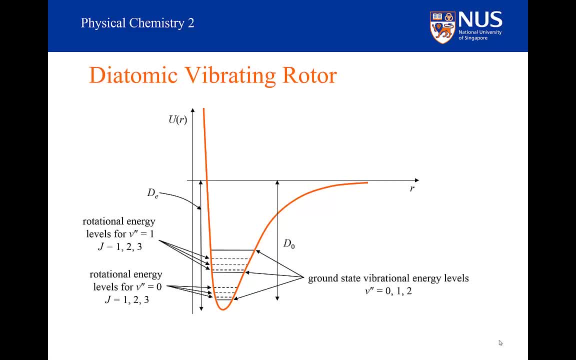 Molecules in these levels up here have vibrational energy associated with v equals one, But they have different values of j: j equals one, j equals two and j equals three. again, The really important thing you want to note is that we can define any of these levels. 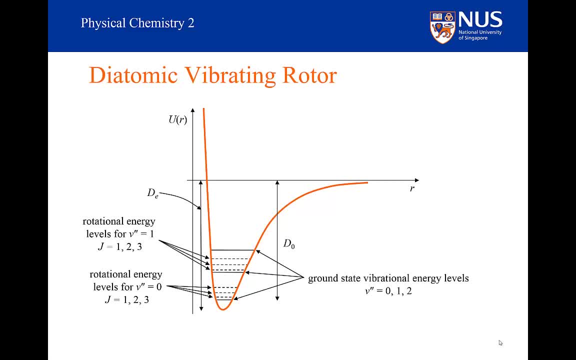 whether it is solid or dashed by two quantum numbers. I know they are in a particular electronic state, So the electronic state is just defined by the potential function. So, given this electronic state, I only need two quantum numbers to define the energy of a particular molecule. 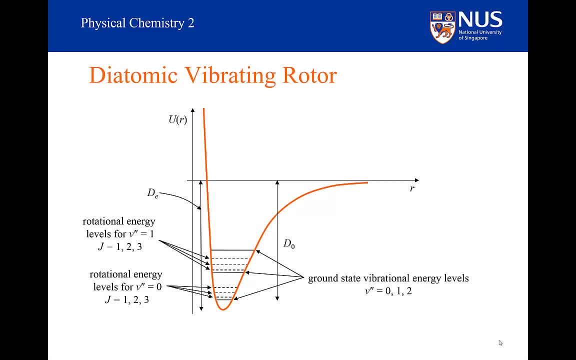 Its vibrational quantum number and its rotational quantum number, Because once I've got these two numbers, I know how much rotational energy it has and I know how much vibrational energy it has, And if I want to know its total energy, I can just sum it together: 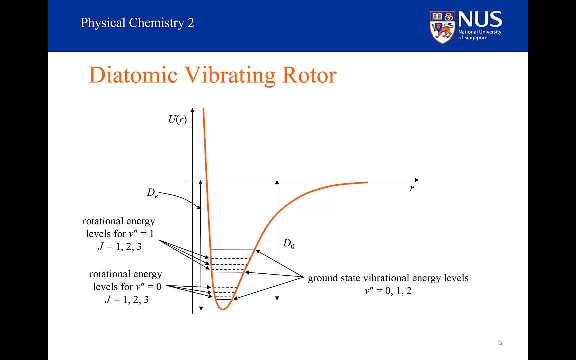 And that's the basis of spectroscopy. Once I know the energies of any levels and I've got my selection rules which tells me how my v can change and how j can change, I can say what transitions are allowed in my system and I can predict the spectrum. 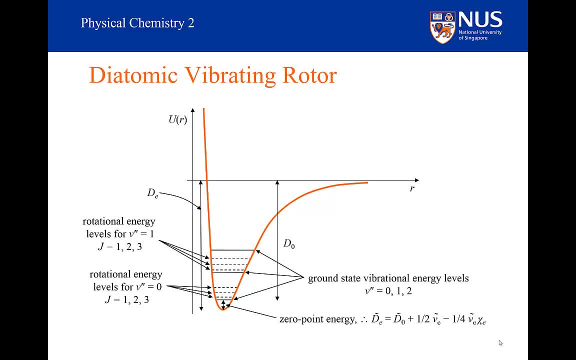 Between the bottom of the potential energy well and the state identified by, v equals zero, j equals zero, we have our zero point energy, which means that I can write dE in terms of d zero. dE will be d zero plus our zero point energy. 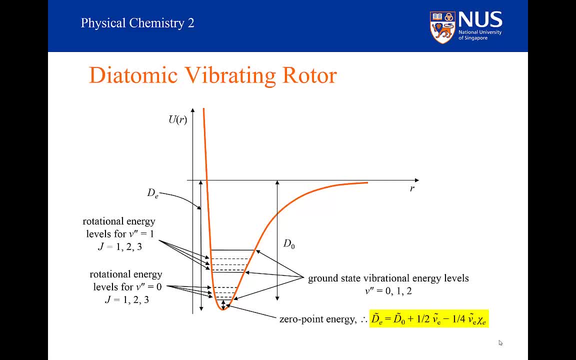 Which is just the energy of our v equals zero state. That is, a half nu E minus a quarter nu E chi E. So when we excite a molecule from one vibrational state to another, we predict that there will also be a change in the rotational state. 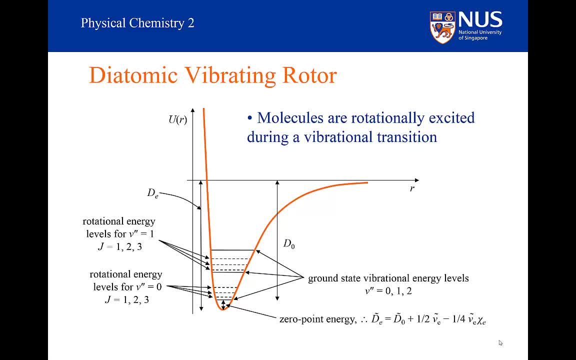 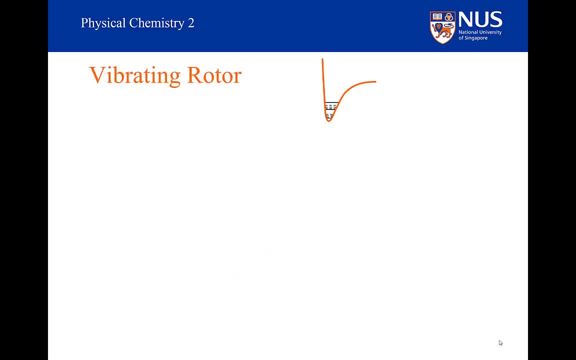 The molecule will be either rotationally excited or de-excited during the row vibrational transition. I've drawn out the potential energy again, But I want to focus on the v equals zero and v equals one state and expand it. This is the energy level diagram again. 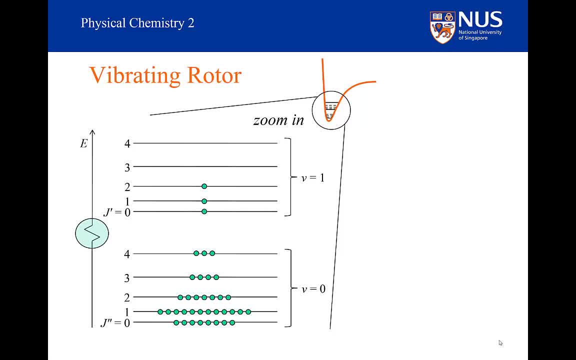 and I've written this zigzag here to illustrate the big gap in energy between the energy levels associated with v equals zero and those associated with v equals one. All the levels identified with the v equals zero quantum number have exactly the same amount of vibrational energy. 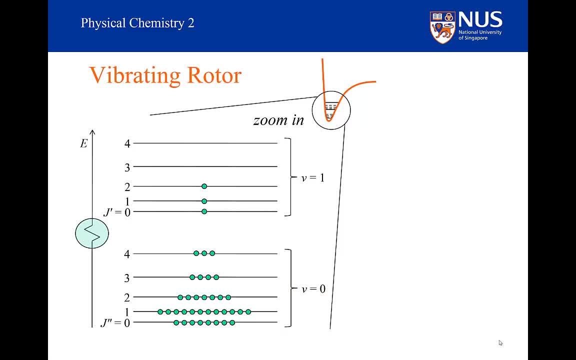 a half nu E minus a quarter nu E, chi E. And all the levels identified with the v equals one quantum number have exactly the same amount of vibrational energy, that is, three halves nu E minus nine quarters nu E, chi E. Both of the energy levels labelled by j equals two. 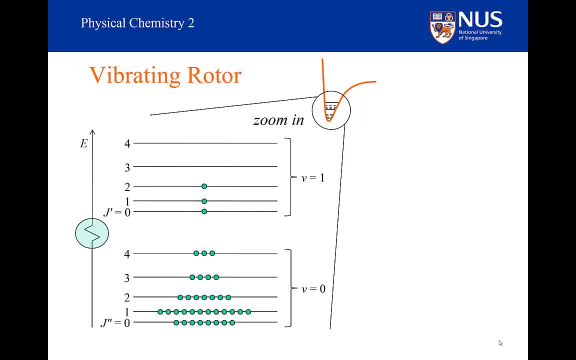 have pretty much the same rotational energy. The reason why it doesn't have exactly the same is because, as you go to higher and higher vibrational energy levels, the bond length is going to change slightly due to anharmonicity. And because the bond length changes, 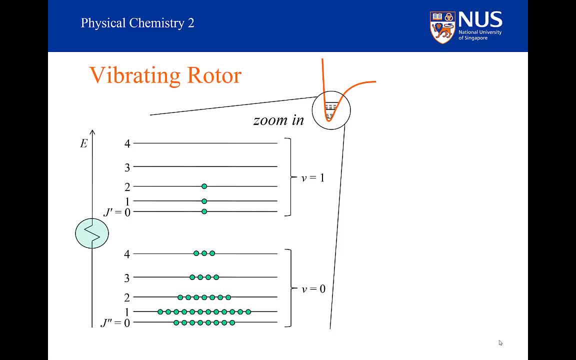 it means the rotational constant changes and remember, the rotational energy is going to be proportional to the rotational constant. So it's not quite the same rotational energy, but it's almost the same. The bottom line is, if I know v and I know j, and although there is a little bit of coupling between the two, 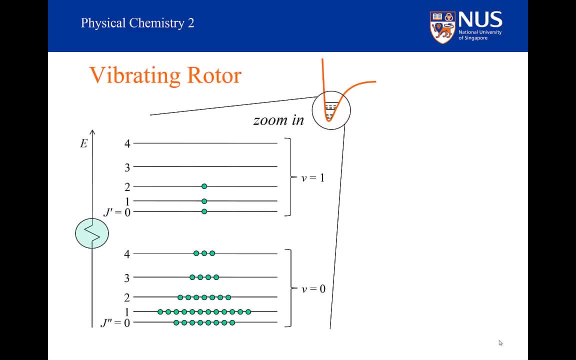 in the way I've just described, I can determine exactly what the energies are for all of these energy levels. When I excite a molecule from an energy level associated with v equals zero to one associated with v equals one, it can either increase its rotational energy. 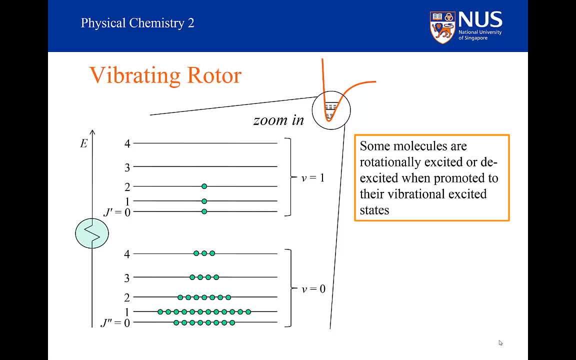 or decrease its rotational energy. We either excite it or de-excite its rotational energy. when we vibrationally excite the molecule, I've tried to illustrate the Boltzmann distribution we expect for our molecules in the v equals zero energy level. Notice that I've put more molecules in the j equals one state. 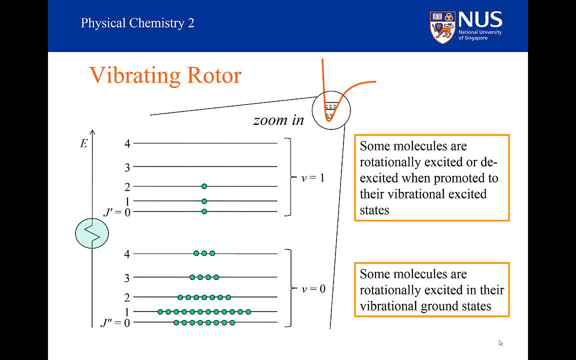 because, remember, rotational levels are degenerate. the level of degeneracy increases as 2j plus one and, as I've stated before, the more levels you've got with a particular energy, the more chances you've got to have molecules in those levels At thermal equilibrium. 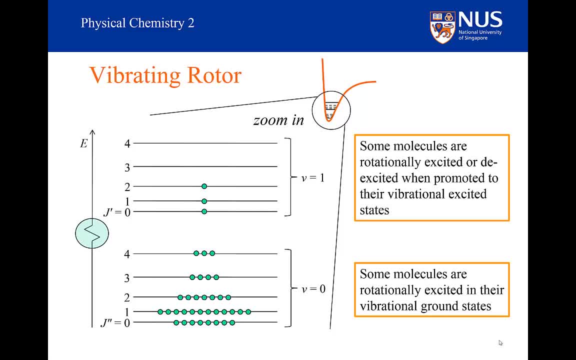 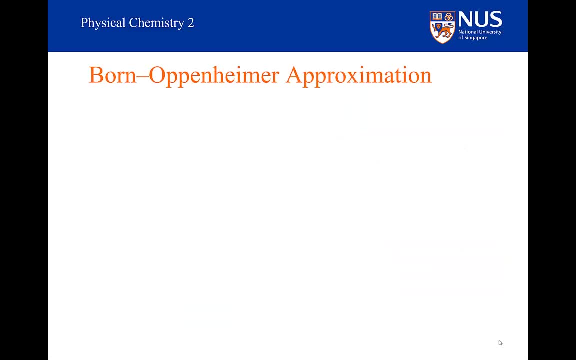 this may well be the kind of population in each of the rotational levels associated with v equals zero. It is clear that during a vibrational transition we are going to have transitions from a large number of initial j states. The Born-Oppenheimer approximation. 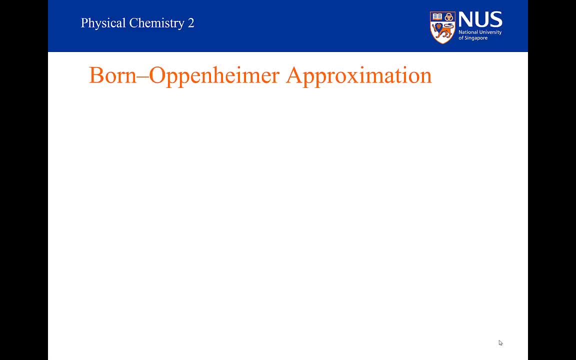 is something you may have heard of before. This is a way of separating the electronic energy from the vibrational and rotational energies. Imagine that I stretch a bond in the molecule. what happens to the electrons? Do they stay where they originally were or do they move? 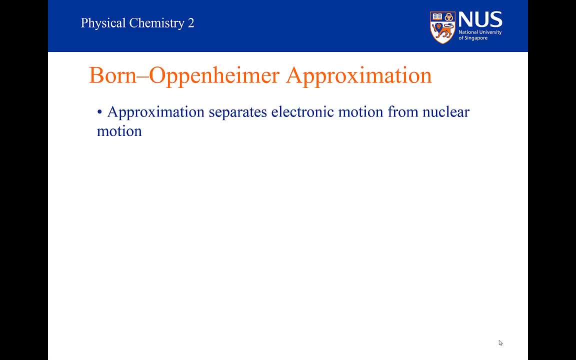 Because of the difference in energies and the difference in mass of the electrons and the nuclei. what happens is that the electrons change instantaneously. compared to the speed with which the nuclei are moving, They adjust themselves instantaneously. It enables us to discuss vibration and rotation. 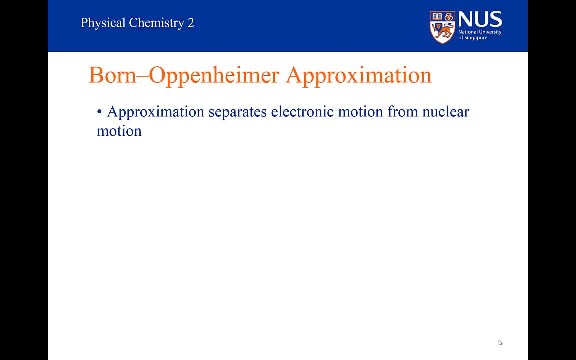 independently to the electrons themselves. So we can just consider the molecule rotating and vibrating in the potential energy. well, We can assume that the potential energy well doesn't adjust because of the vibrations and rotations, and it is an incredibly good approximation. Further, because of the differences in energies, 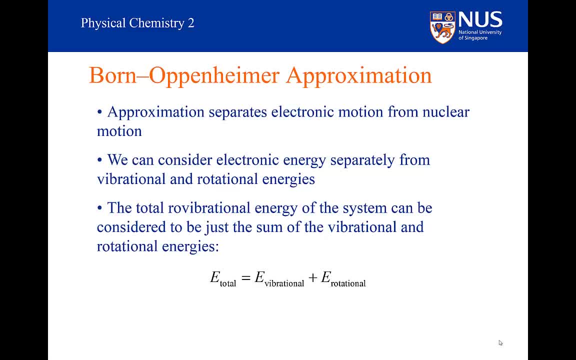 we can largely separate the vibrational energy away from the rotational energy as well and just consider the total row vibrational energy as the sum of the vibrational energy and the rotational energy that we would calculate from the vibrational problem and the rotational problem separately. 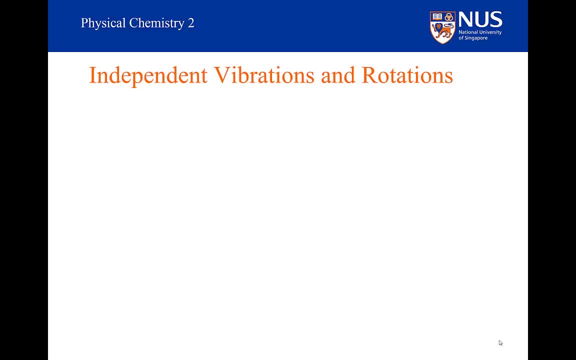 Although I have already mentioned that there is some coupling between the vibrations and rotations, let's start by considering them to be independent. So we will ignore centrifugal distortion to reduce the amount of energy and the amount of mass. We can always include it later. 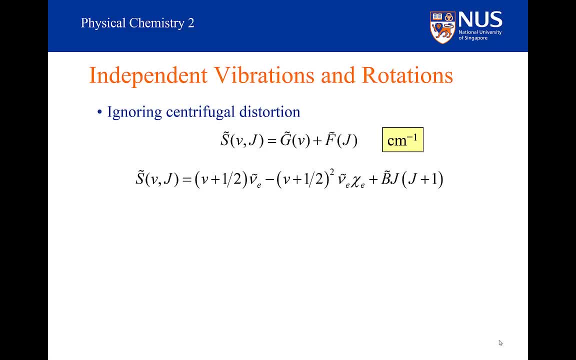 If I want to know the energy of a molecule that is in the V vibrational state and the J rotational state, it literally is just the vibrational energy plus the rotational energy, And I can write out our vibrational term and rotational terms like so so that the total energy. 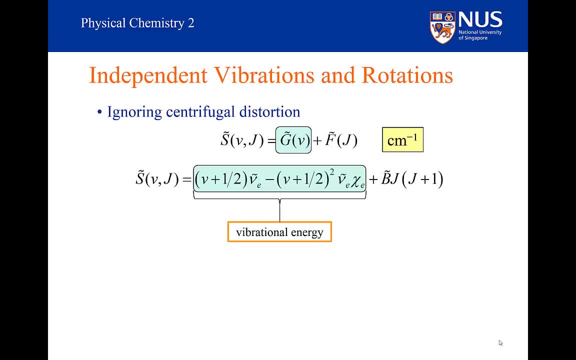 or row vibrational energy is going to be V plus a half nu E minus V plus a half. squared nu E, chi E plus B, times J into J plus 1.. The total amount of energy is just the sum of the vibrational energy and the rotational energy. 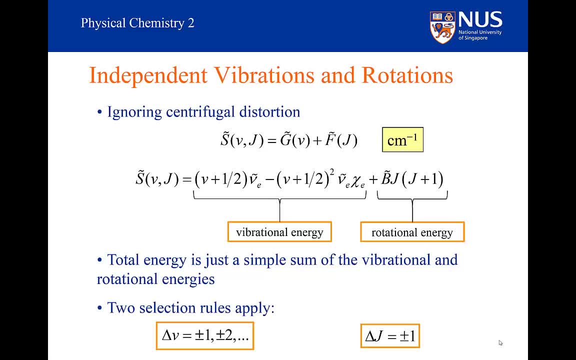 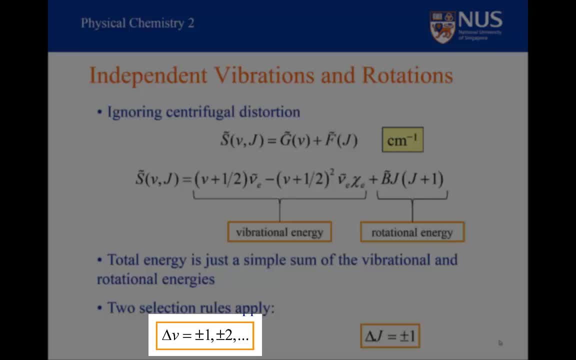 To predict the spectrum that will result from row vibrational transitions, we need to take into account both the selection rules. Delta V can be plus or minus 1, or plus or minus 2, etc. But of course transitions for delta V greater than plus or minus 1. 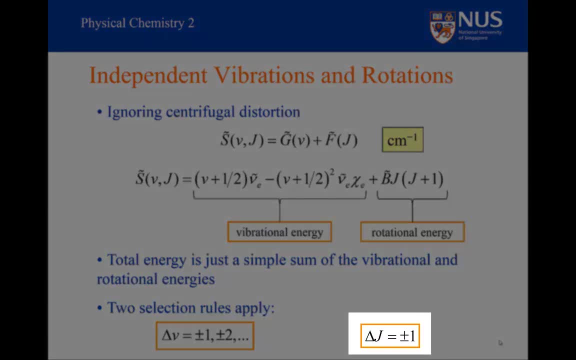 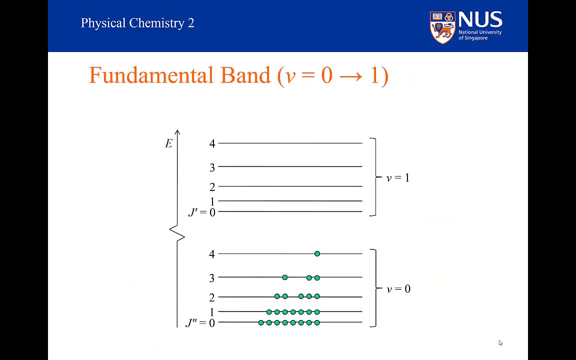 will exhibit far weaker spectral line intensities, and that delta J is equal to plus or minus 1.. Let's see how this affects things. Let's draw out our row vibrational energy levels once more. We are going to look at just the fundamental band. 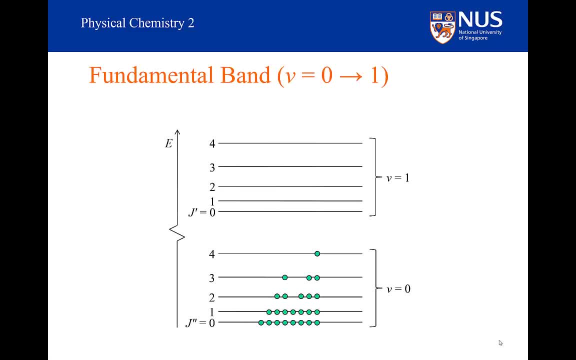 in which we excite molecules from V equals 0 to the V equals 1 state, But delta J has to be equal to plus or minus 1.. What does this mean? It means that I can get transitions like this: from J equals 0 to J equals 1. 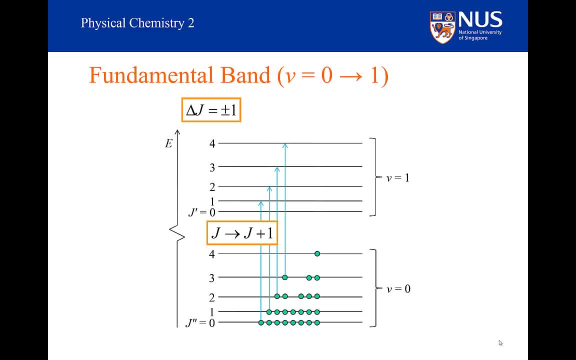 or J equals 1 to J equals 2, or J equals 2 to J equals 3, or J equals 3 to J equals 4, etc. Or I can get transitions like this: from J equals 1 to J equals 0, J equals 2 to J equals 1. 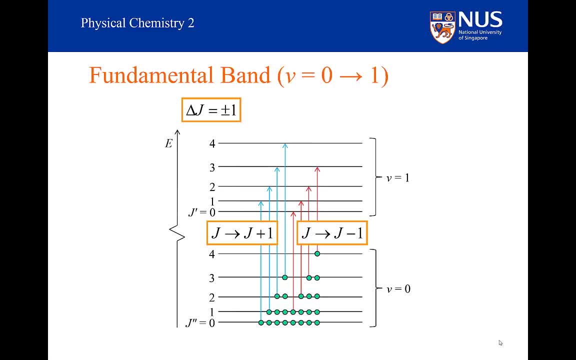 J equals 3 to J equals 2, and J equals 4 to J equals 3, etc. So I can have these blue transitions where J is increased by 1 and I can have these red transitions where J is decreased by 1.. When J is increased by 1: 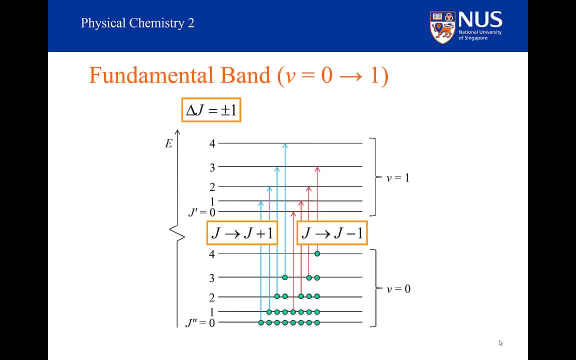 we identify these transitions as R branch transitions. Notice that all these transitions where J has increased will be at a frequency that is larger than the fundamental frequency. The fundamental frequency can be identified in a hypothetical transition in which J doesn't change When J has decreased by 1. 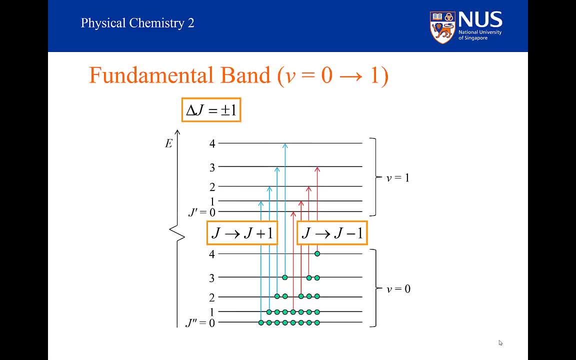 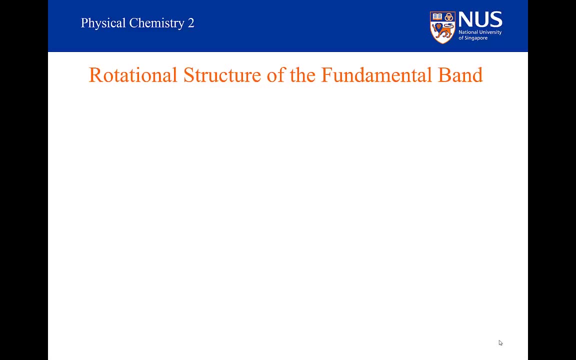 we identify these transitions as P branch transitions. Notice that all of these transitions where J has decreased will be at a frequency that is smaller than the fundamental frequency. So let's use our knowledge of the vibrational and rotational energies and the selection rules to predict transitions in the P branch. 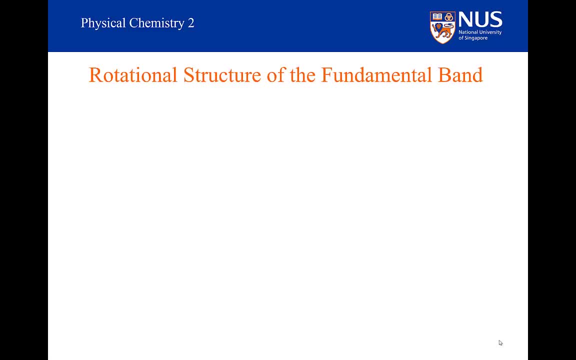 where J decreases by 1, and in the R branch, where J increases by 1.. So for the P branch the rotational state changes from J double prime to J prime. The double prime indicates the initial state and the single prime indicates the final state. 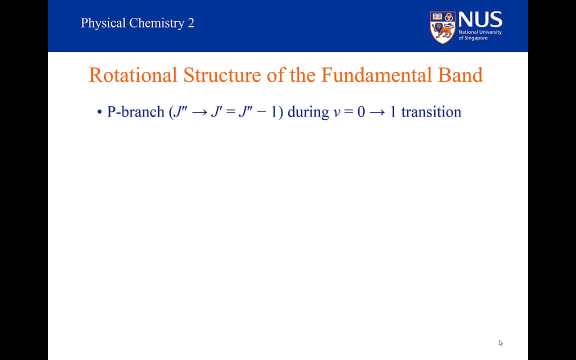 This is purely a convention. So if my initial state is J double prime, then my final state is related to my initial state, because J prime will be equal to J double prime minus 1.. The rotational state has decreased by 1, which is the definition of a P branch transition. 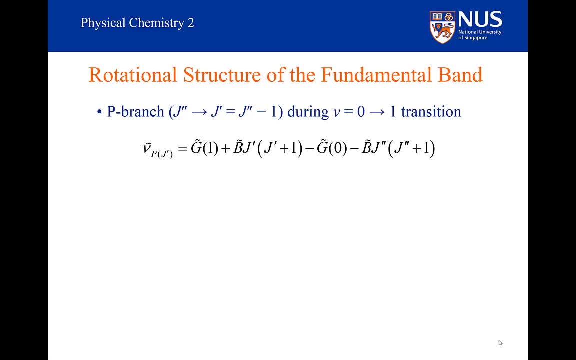 This means that I can write down the frequency of any line in the P branch. Here is the total row vibrational energy of the final energy level And here is the total row vibrational energy of the initial energy level, which I am subtracting to find. 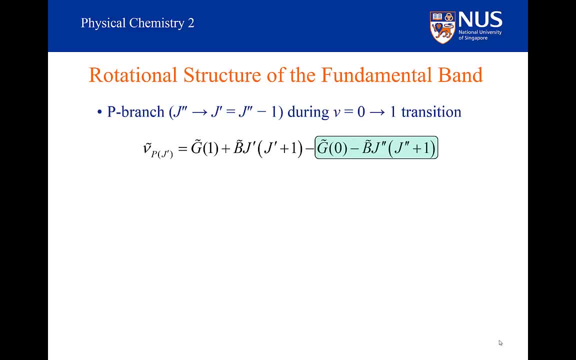 the difference, which will be the frequency of the spectral line. Now I can rearrange this equation here and write: by substituting J double prime is equal to J prime plus 1, which is the relationship for the initial and final rotational states for a P branch transition. 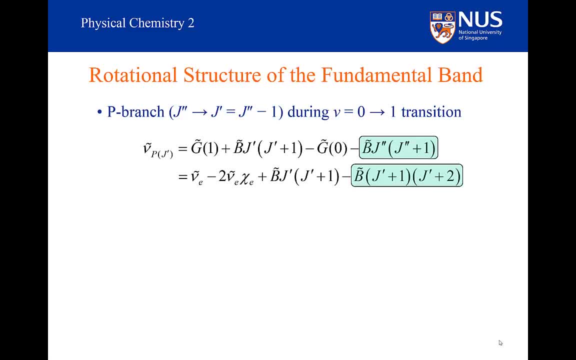 Therefore I can substitute for J double prime in the rotational term for the initial state with J prime plus 1. The result is B into J prime plus 1 into J prime plus 2. So you just simply substitute into this equation and you get this. 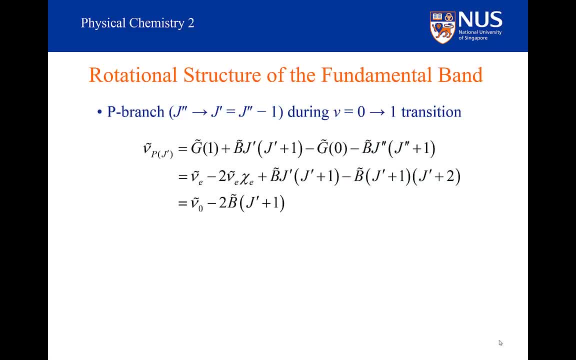 We can now simplify this expression and this is what we get: B into J prime, into J prime plus 1, minus B into J prime plus 1 into J prime plus 2 will just be 2B into J prime plus 1.. So we have our fundamental frequency. 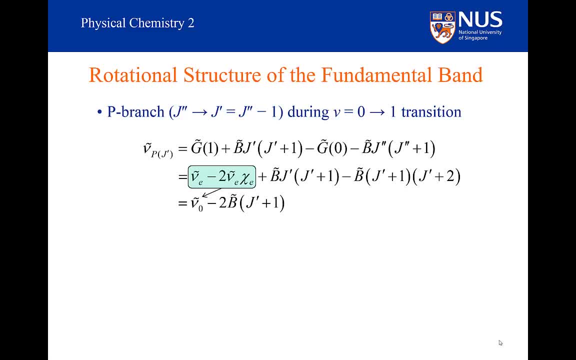 which is nu zero minus the result from the difference in the rotational energies, that is 2B, into J prime plus 1.. We can do exactly the same for the R branch. In the R branch I go from J double prime to J prime again. 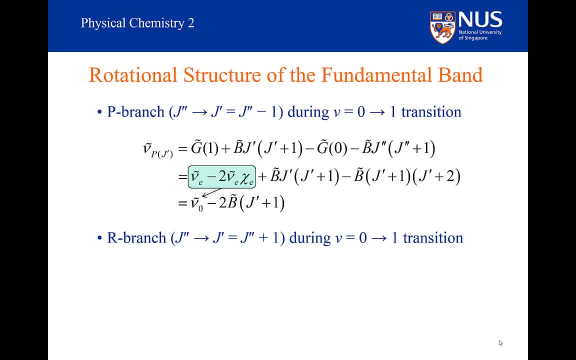 but I can write J prime in terms of J double prime, because for the R branch J goes up by 1. So therefore J prime must be equal to J double prime plus 1.. Once again, I can write down the frequency of a transition in the R branch. 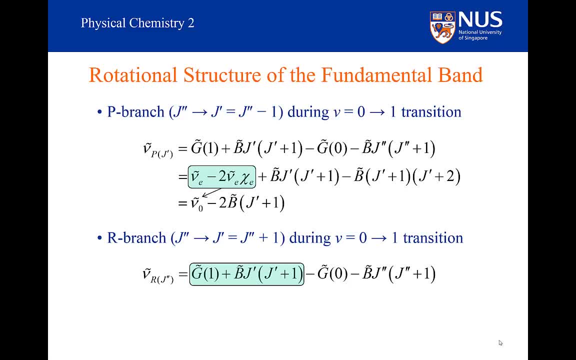 as the difference between the row vibrational energy in the final state and the row vibrational energy in the initial state. This time I will substitute J prime, so I substitute in J double prime plus 1 into this equation And therefore I will get an expression. 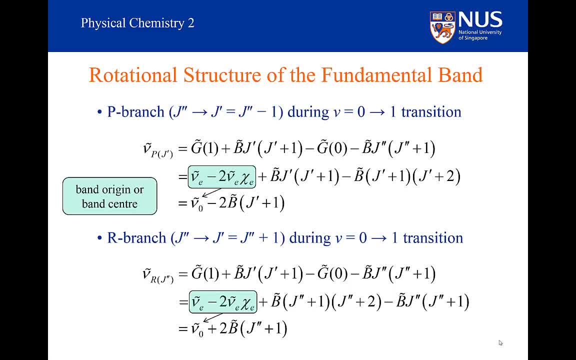 that will look like this: We have nu zero again, because this is my fundamental frequency, plus the term 2B into J, double prime plus 1.. So there are two differences here between P and R branch lines. In the P branch the difference between 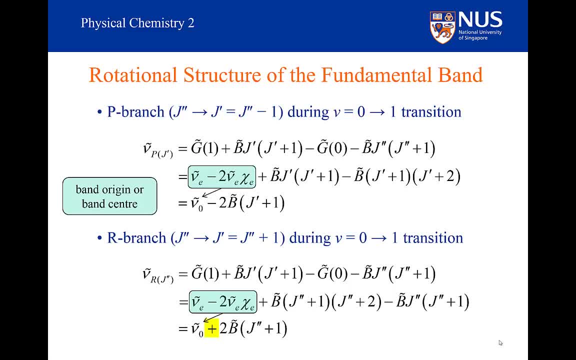 the rotational energies is negative, but in the R branch it is positive. In the P branch, I define it in terms of J prime, the final J value, and in the R branch in terms of J double prime. This is solely to show the similarity between the expressions. 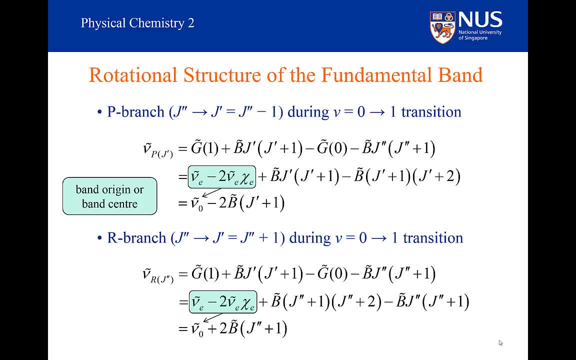 Note that we never get a transition at exactly the fundamental frequency. These two equations define all the possible spectral lines in the P branch and in the R branch. There are no other branches for the diatomic. For the P branch, the minimum value of J prime is zero. 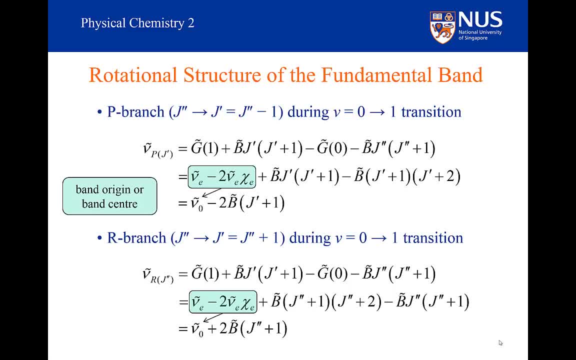 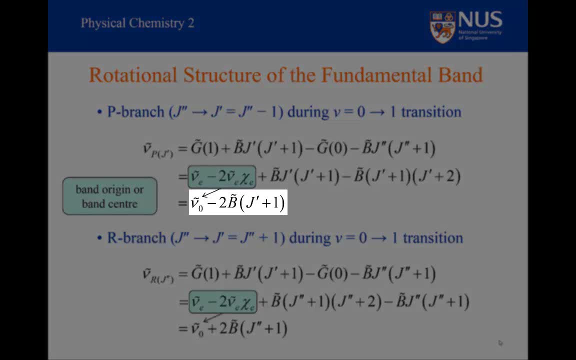 It can't be lower than zero. You can go from J equals 1 to J equals zero. So the minimum value of J prime is zero, and if you substitute this into this equation, the first line in the P branch will be at nu zero minus 2B. 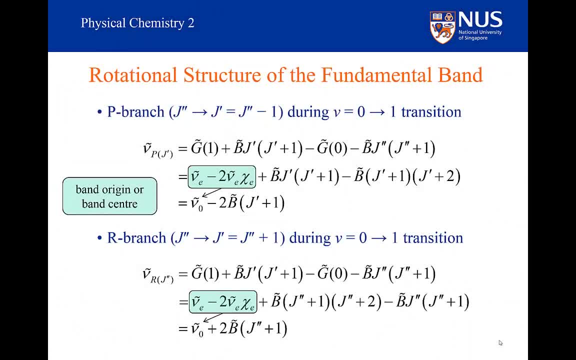 Again, the minimum value of J double prime is zero as well. Therefore, the first line in the R branch will be at nu zero plus 2B. This means there's going to be a gap of 4B between the first line in the R branch. 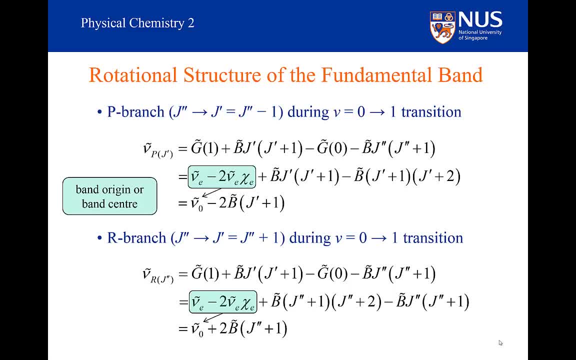 and the first line in the P branch And in the middle of that gap is going to be the fundamental frequency. So this enables us to easily identify what the first line in the P branch is and what the first line in the R branch is, because all we need to do 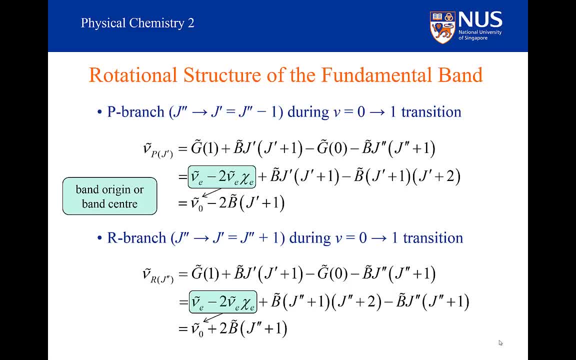 is find that gap. Once we've found that gap, we know that the lines at smaller frequencies are P branch lines and the lines at higher frequencies are R branch lines. Note that the centre of this gap associated with nu zero is referred to as the band origin. 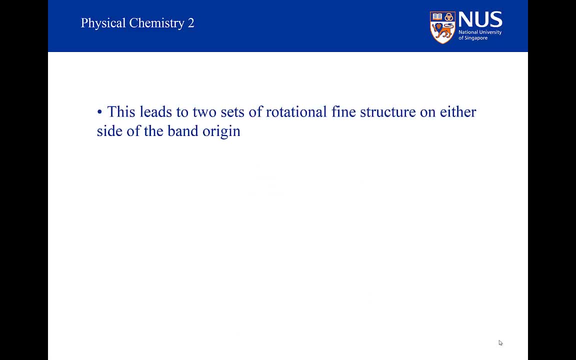 or band centre. So we've got two sets of rotational fine structure on either side of the band origin, exactly what we saw for the carbon monoxide spectra. And notice that I can also write the P branch in terms of J prime or J double prime. 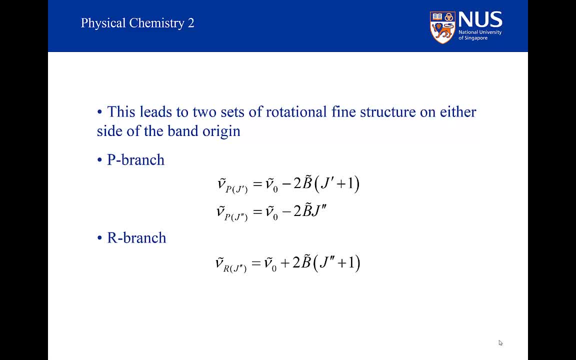 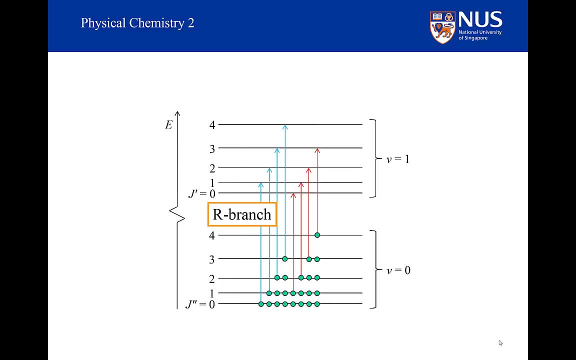 And here is the expression once again for the R branch. So these are the transitions that we've seen. We've got the R branch over here and we've got the P branch over here. So now that we know what the frequencies are for the P branch, 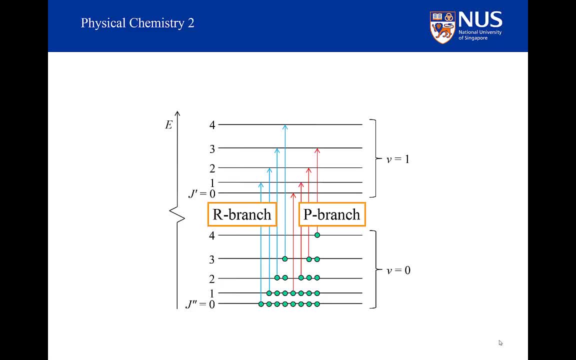 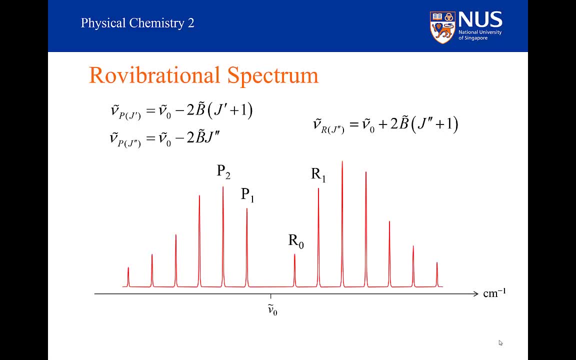 and for the R branch spectral lines, we can predict the structure of the Rho vibrational spectrum. Here is the Rho vibrational spectrum predicted by our expressions for the spectral line frequencies for transitions in the P and R branches. Note the gap I spoke about. 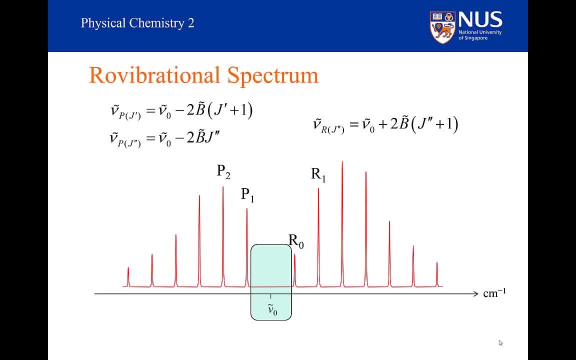 which occurs at the fundamental frequency. The first line at higher frequencies is part of the R branch and we identify it as R zero because it is associated with the J equals zero to J equals one transition. The first line in the P branch at lower frequencies. 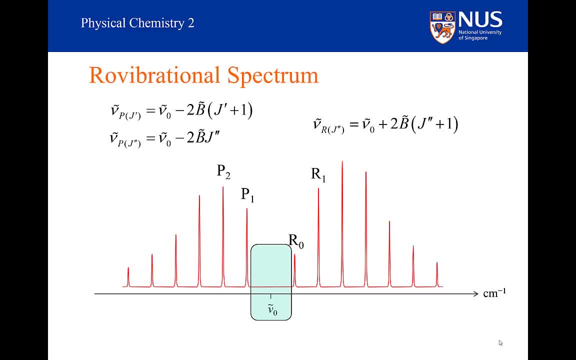 is labeled as P one, because you're going from the J equals one state to the J equals zero state, So the number refers to the initial level. This type of convention is consistent throughout spectroscopy- The numbers that we generally use when we try to label a spectral line. 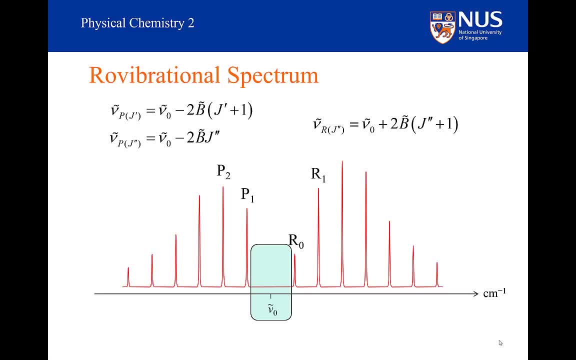 refer to the initial state. So the line labeled R zero is for the transition from J equals zero to J equals one, and the line labeled R one is for the transition from J equals one to J equals two, etc. Similarly, in the P branch the line labeled P one. 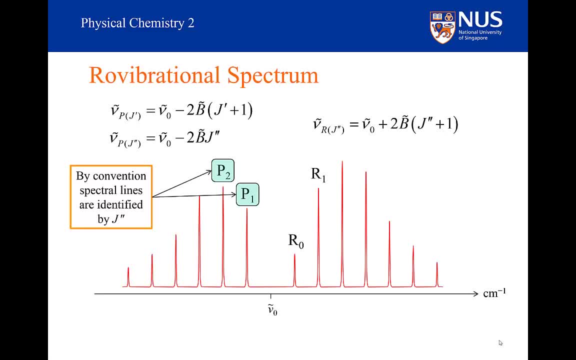 is for the transition from J equals one to J equals zero, and the line labeled P two is for the transition from J equals two to J equals one, etc. The number again identifies the initial rotational level. We can also see that in this analysis, where we have ignored centrifugal distortion. 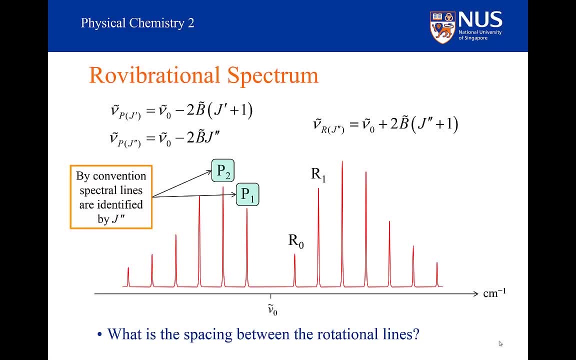 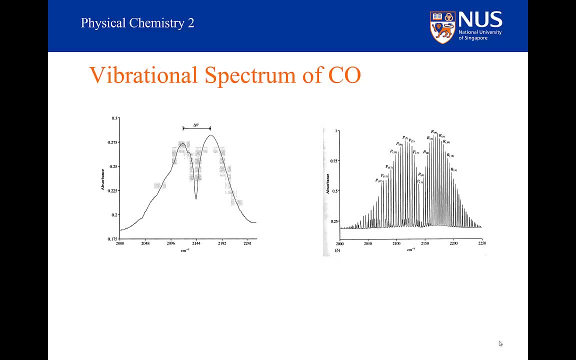 the spectral lines are evenly spaced and you can see that the difference between any two adjacent spectral lines, ignoring the gap at the band origin, is just going to be two B. So this explains the vibrational spectra of carbon monoxide that I introduced in part one. 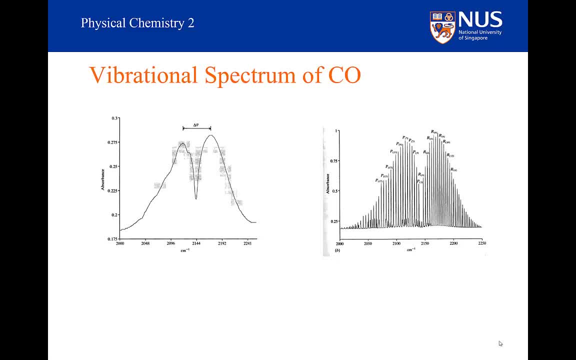 We've now accounted for both observation three and observation four. With observation three the low resolution of the spectrometer averages out the fine rotational structure so that we see two broad bands associated with the unresolved P and R branch spectral lines. But at high resolution we can see the rotational structure. 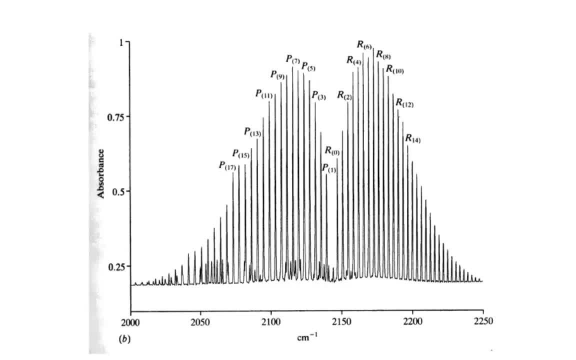 and we can see the fact that these are evenly spaced lines, as predicted earlier. So you can see here the R zero, R one, R two, R three and R four spectral lines. Similarly the P one, P two, P three spectral lines, etc. 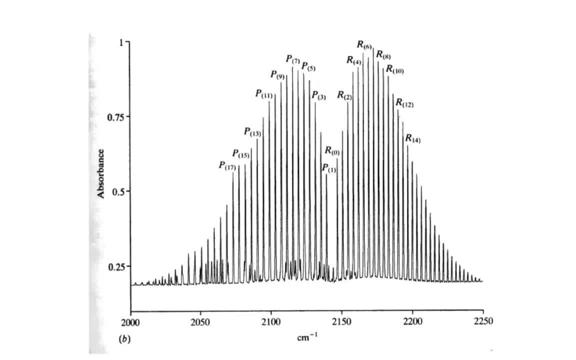 So you can see how easy it is to label our lines. You just find the band centre. The first line at the lower frequency is P one and the first line at the higher frequency is R zero. You can know exactly what the J quantum numbers. 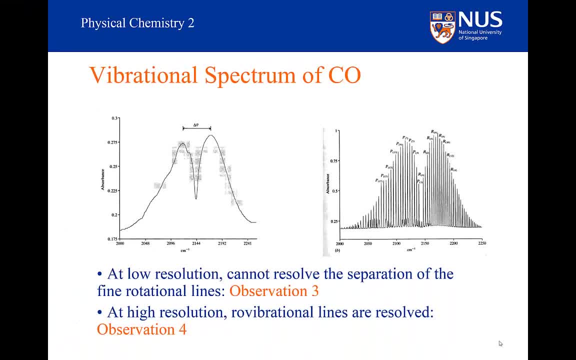 of all the lines are. I just want to emphasise this once more. The picture that I am trying to imprint in your mind is this idea that the quantum mechanics gives us two things: It enables us to define a level with quantum numbers and, if I know the quantum numbers,